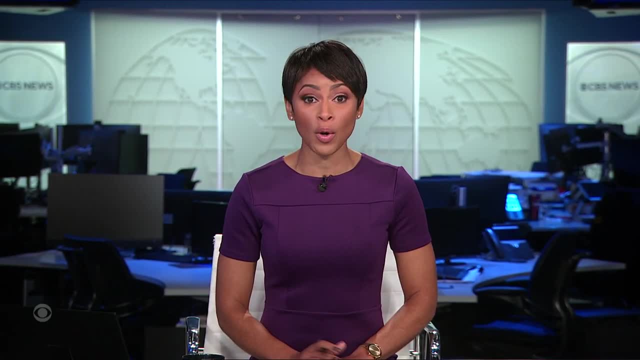 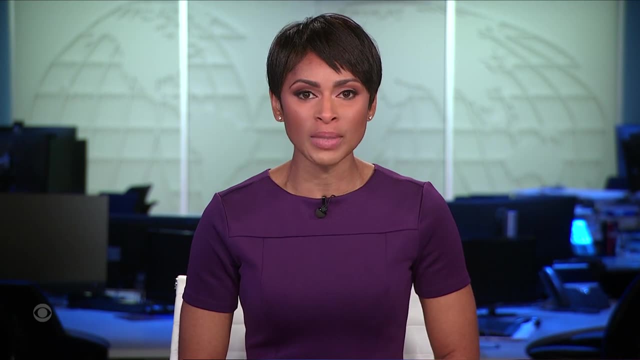 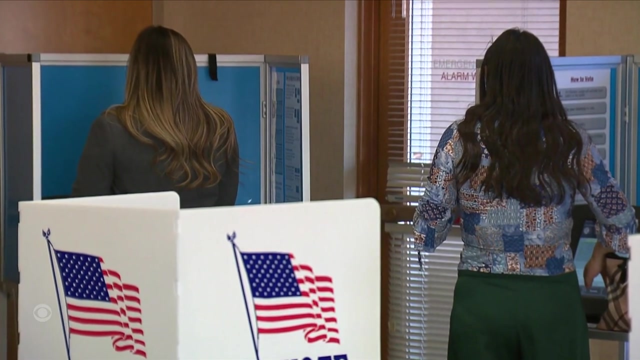 We begin tonight with the fast approaching midterm elections. Both parties are pressing hard to show why they deserve your vote. Democrats focused on their legislative accomplishments, Republicans on the economy and crime. At stake, both houses of Congress. Votes are already being cast in many states across the country, in person and by mail. CBS's Christina Ruffini leads us off. 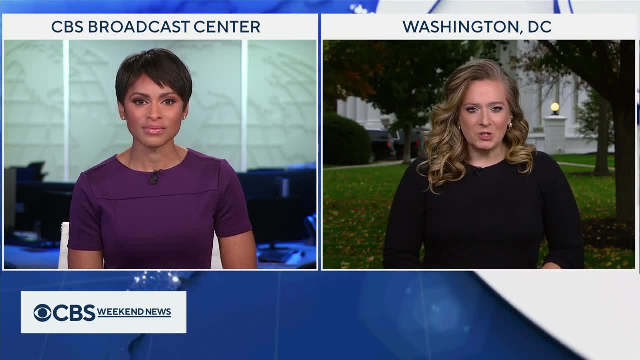 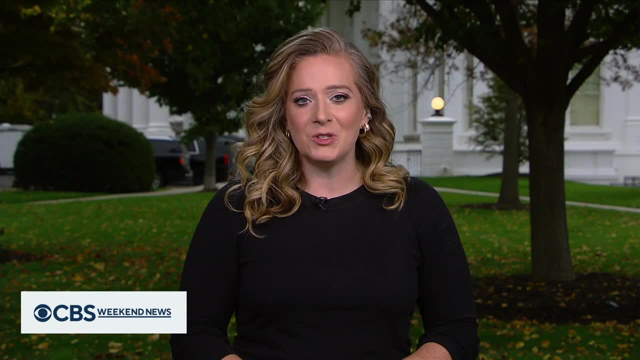 tonight from the White House, Christina. good evening, Good evening Jerika. Well, after a quiet weekend at home in Delaware, President Biden will head to Pennsylvania this week and Florida the next, as we come into the home stretch of this contentious midterm election. 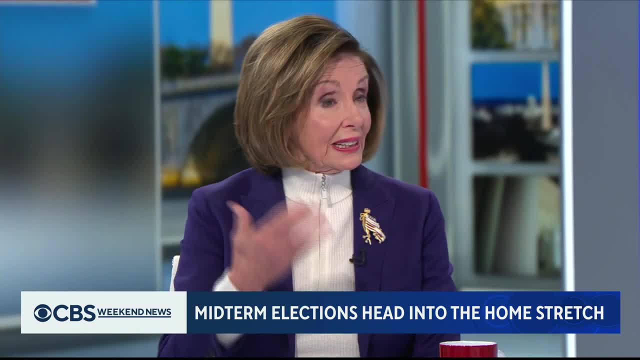 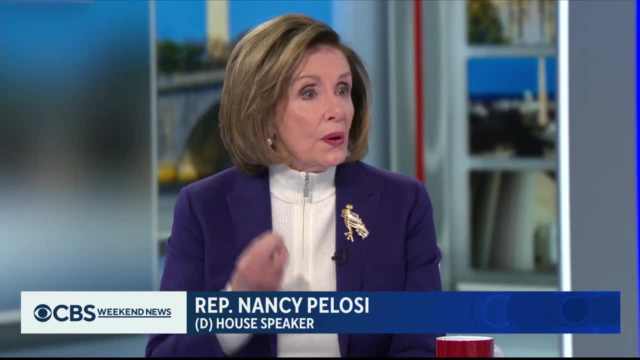 These are tough fights On Face the Nation. today, Speaker of the House Nancy Pelosi said the results of the midterms will be decided in the last minutes of the race. I see very clearly that the ownership of the ground is with us, But the latest CBS News battleground tracker poll: 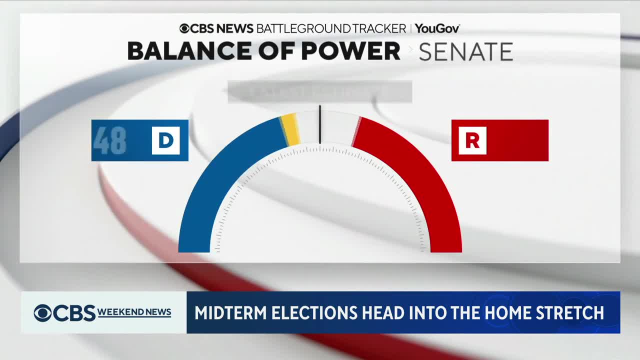 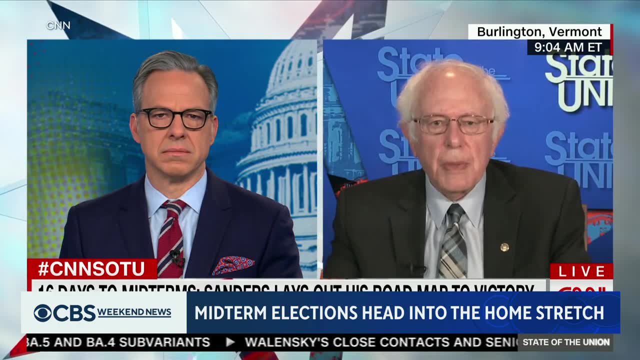 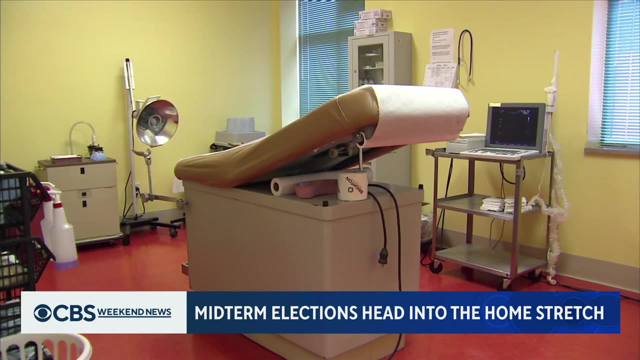 has the House likely going to the Republicans and the Senate at a 50-50 split? I am worried about the level of voter turnout among young people and working people, who will be voting Democratic. The surge of support Democrats saw over the summer following the overturn of Roe v Wade has faded. 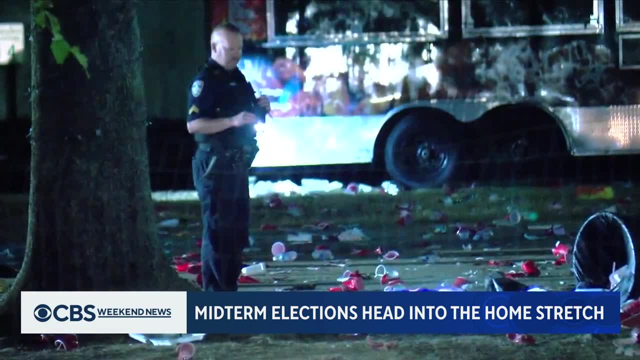 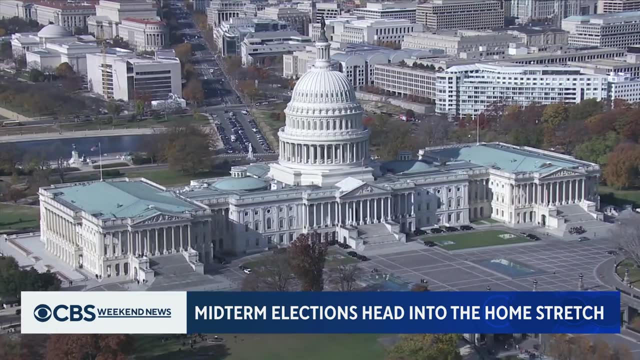 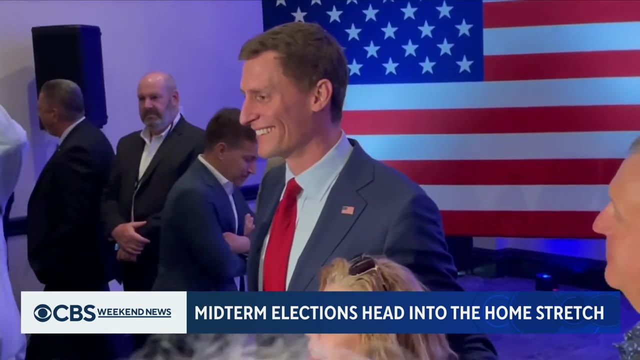 Crime is going through the roof, As Republicans are trying to focus voters on issues like crime, immigration and the economy. This is an economic and health crisis. In several key races, including the tied-up Arizona Senate, Republican candidates have openly questioned the results of the 2020 election. 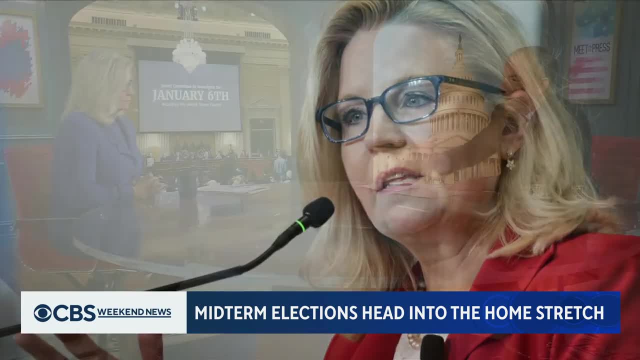 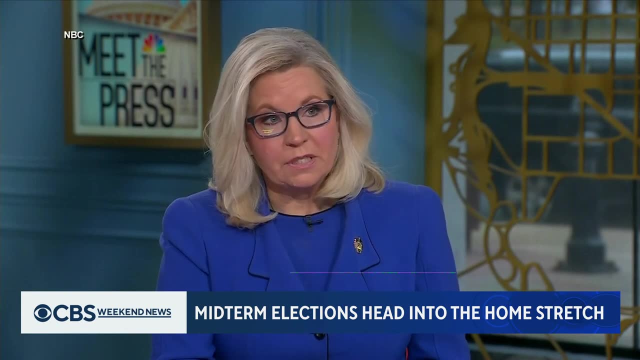 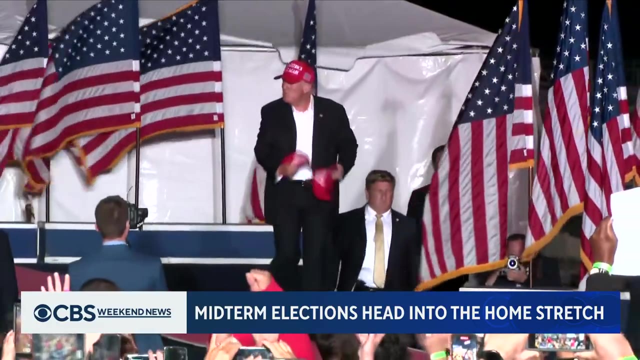 I think Trump won in 2020.. Today, House Republican Liz Cheney warned that election deniers are a threat to democracy. No one of any party should be voting for people who are election deniers. I ran twice, I won twice, But at a rally in Texas last night, former President Trump repeated his usual false claims. 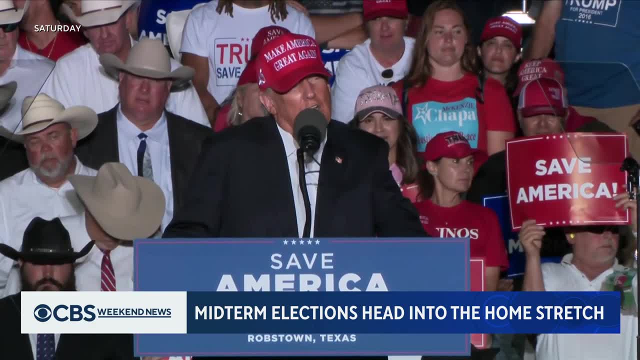 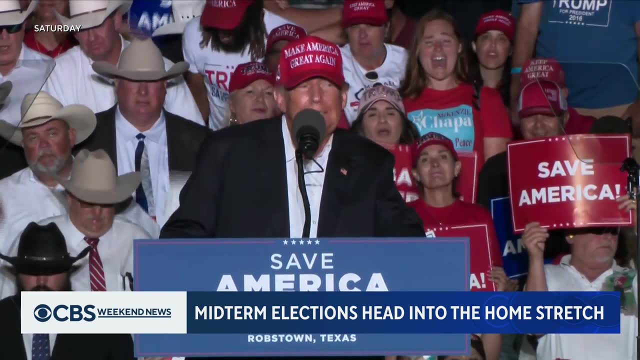 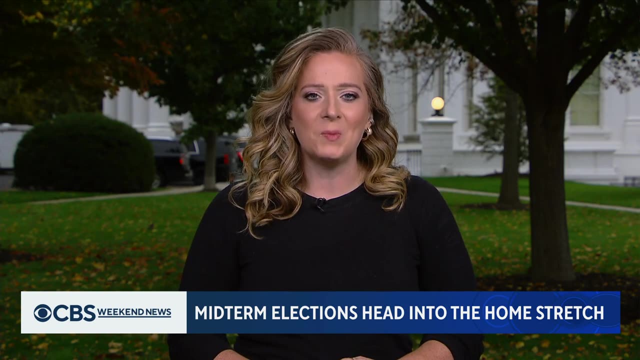 then teased another run In order to make our country successful, safe and glorious again. I will probably have to do it again, And President Biden said in an interview this weekend that he could run again in 2024, but he won't make that decision officially until after the midterm elections. Jerika Christina, thank you.